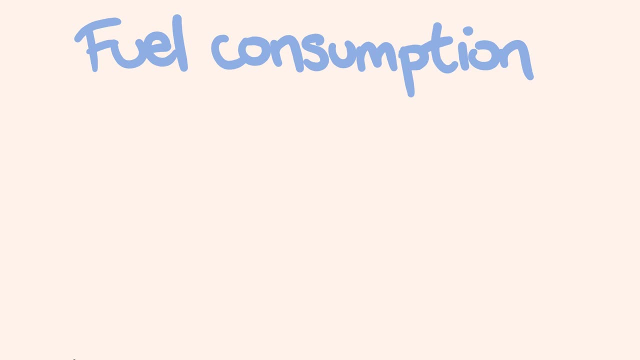 a given distance and it can be measured in a number of different ways. We can measure it in terms of the number of kilometers you could drive with one litre of petrol, the kilometers per litre. We could also look at the number of litres you would use to drive 100 kilometers. that is the 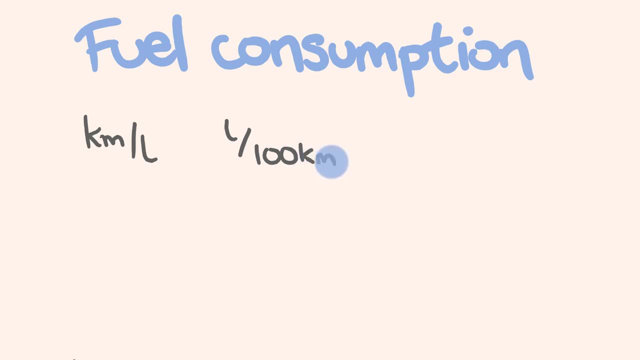 litres per 100 kilometers. We could also use the number of miles that you could go per gallon- miles per gallon- And you're going to notice for each of these that we actually have a formula that we've written out too. We have kilometers divided by the number of litres, and litres 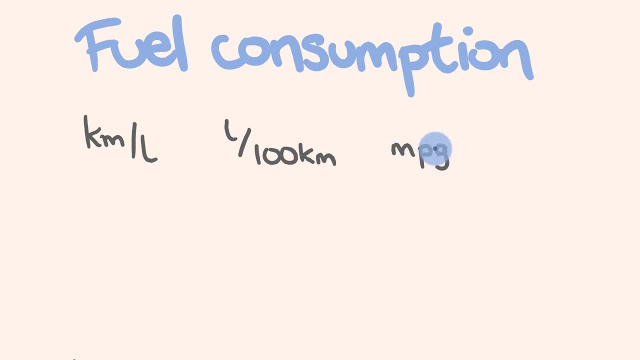 divided by the number of hundred kilometers and the miles per gallon, which means miles divided by the number of gallons, And we're going to be using these to work out a lot of the things to do with fuel consumption. It makes things really really simple. So what about our launch into the first question? So for our first question. 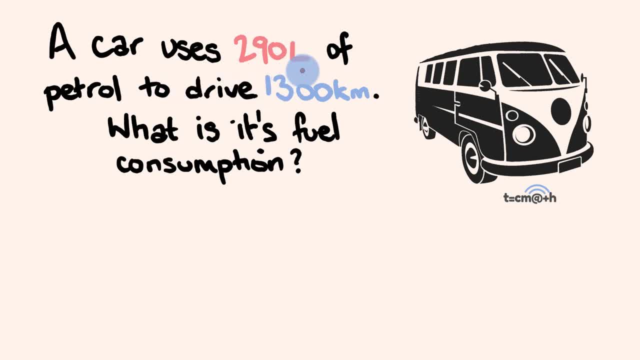 a car uses 290 litres of petrol to drive 1,300 kilometers, What is its fuel consumption? So there's two different ways that we could measure fuel consumption using these particular figures. The first way we can measure fuel consumption is we could say what is the number. 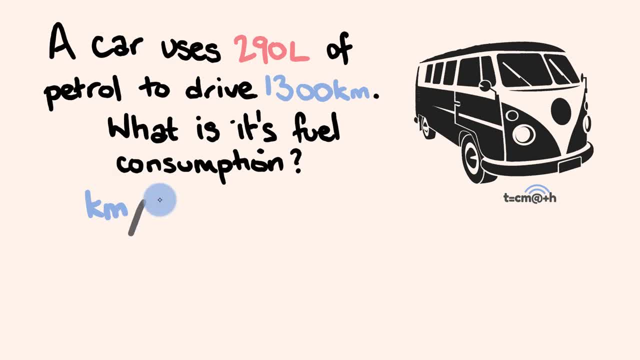 of kilometers that we travel per litre. Okay, the kilometers per litre. The other thing we could do is we could also say: how many litres are we using per 100 kilometers? So we're going to work out both of these, but you might have to specifically work one out. 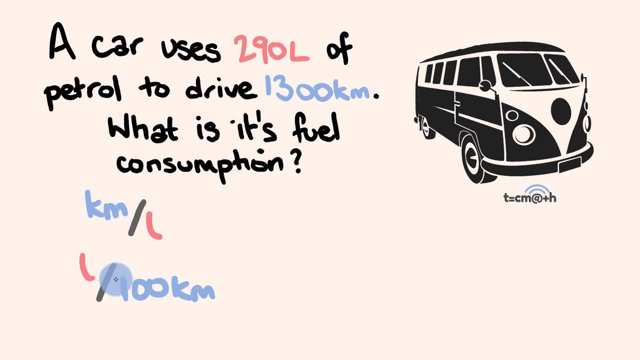 when you were doing this. So we're just going to treat each of our units here as a formula. So we have the kilometers divided by the number of litres. The number of kilometers we have is 1,300 kilometers, and this is going to be divided by the number of litres. This much here. 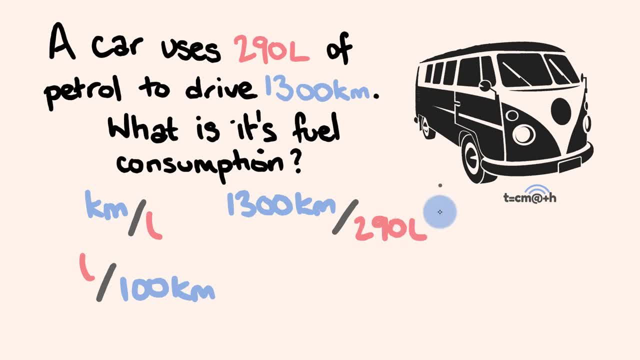 290 litres. Nice and easy, Pretty easy calculation to work out. Okay, and that's going to be 4.5 kilometers per litre. All right, that's the first way. As you can see, I just followed this particular thing: kilometers divided by litres. kilometers per litre. The next one is litres per. 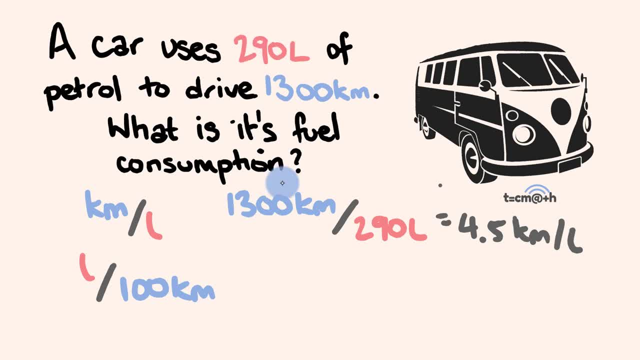 100 kilometers. So let's work this out. We have 290 litres, So let's put that on first: 290 litres, and this is going to be divided by the number of 100 kilometers. As you can see, this is per 100 kilometers. 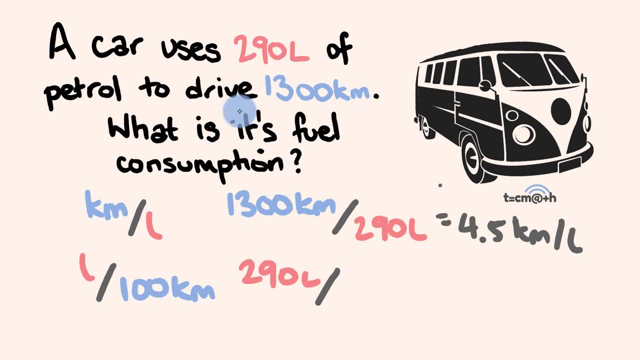 So in 1,300 kilometers, how many hundred kilometers do we have? So 1,300 divided by 100, we're just going to divide that by 13, and we'll get our answer. So 290 divided by 13,. 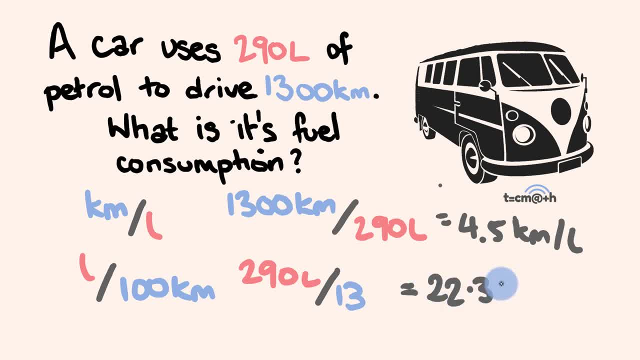 this is going to be 22.3 litres per 100 kilometers, And that's the way that you can work out a fuel consumption really easy. So I'm going to look at this now in terms of miles per gallon. So let's look at this question here. A car uses 43 gallons. 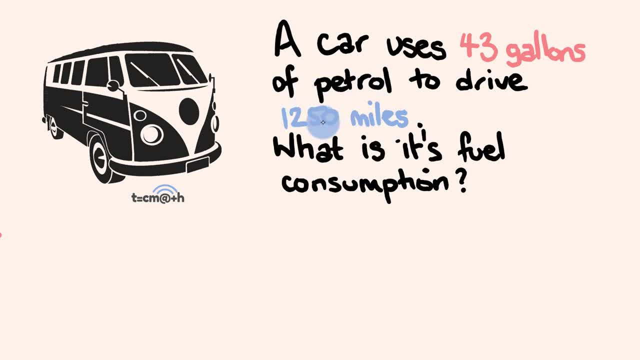 of petrol to drive 1,250 miles. What is its fuel consumption? We've got miles and we're using gallons, So our fuel consumption is going to be in miles per gallon. Okay, and you might think of this as being the per here as actually being divided by, So you can actually see this as the 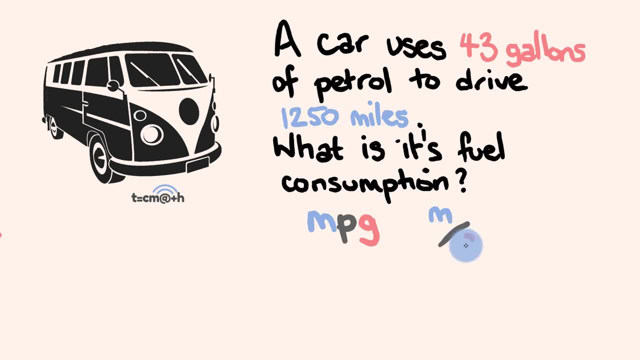 miles divided by the number of gallons. So it's a nice and easy equation to work out. So let's go to. Okay, so let's do this. First off, we have the miles. here We have 1,250, and that's going to be. 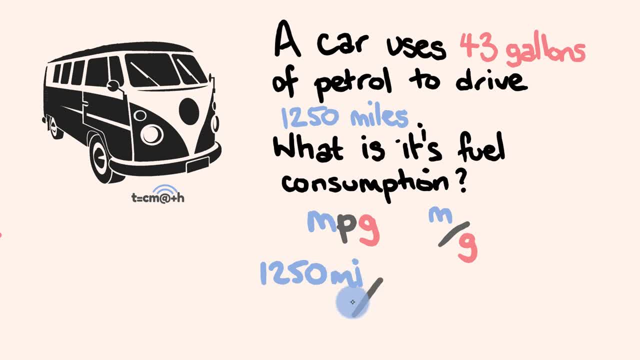 your miles, And this is going to be divided by the number of gallons. We have 43 gallons here, All right, so what do we get when we work this out? 1,250 divided by 43, you're going to get. 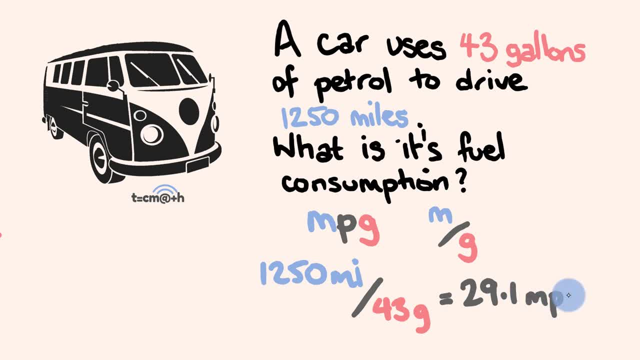 the answer of 29.1 miles per gallon. As I said, nice and simple: Just treat the units that you're working out as an equation, as a formula, and you'll go on from there. Okay, so let's have a look at how then you may apply these once you know your fuel consumption. 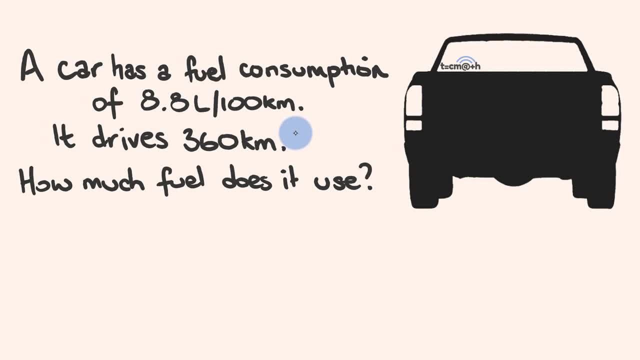 So this is how you would go about applying these. A car has a fuel consumption of 8.8 litres per 100 kilometres. It drives 360 kilometres. How much fuel does it use? So you're going to see here that we have a couple of things. We have the amount of fuel or the amount of petrol. 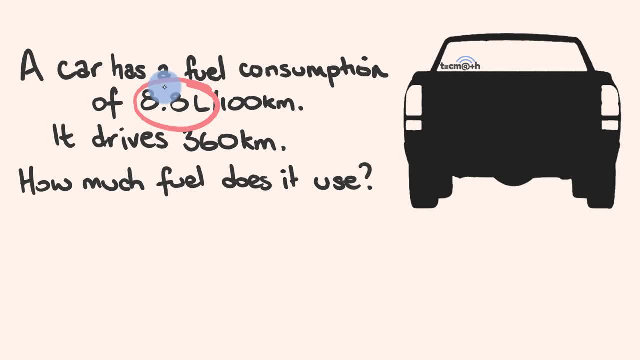 that we're actually we know for the fuel consumption. We've also got this part that we're trying to work out down here. We have 100 kilometres here and we have 360 kilometres that we are travelling, So we're going to be using these to work out proportionally how much petrol. 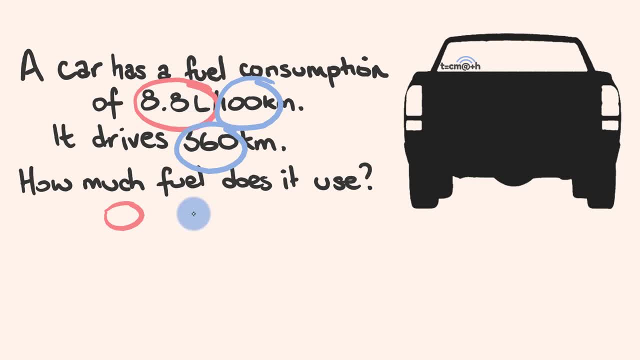 we need Okay, and this is how we're going to do this. So we have 8.8 litres and this is going to take us 100 kilometres, But we don't want to go 100 kilometres, we want to go 360.. 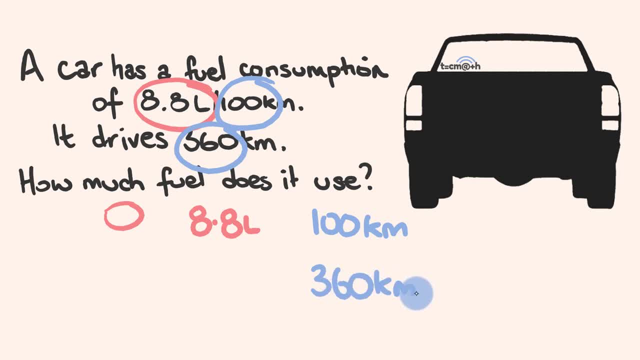 360 kilometres, which is a little bit bigger, And you might say to yourself: okay, how much bigger is it? Because we want to know then how much petrol we're going to use. So how much bigger is 360 than 100? I'm talking proportionally. How much would you multiply 100 by to get 360?? 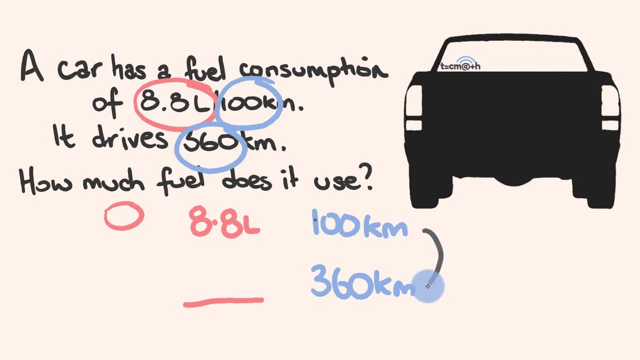 Well, we can go 360 divided by 100 and work that out. So this is going to be multiplied by 3.6.. So we're going to be going 3.6 times as far. We're going to be using 3.6 times as much petrol. 8.8 times 3.6, we're going to have our answer. This is going to be. 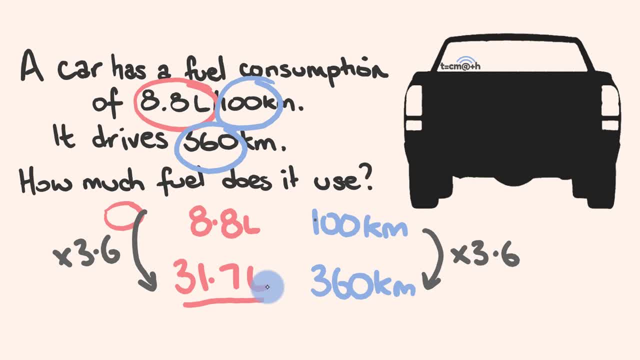 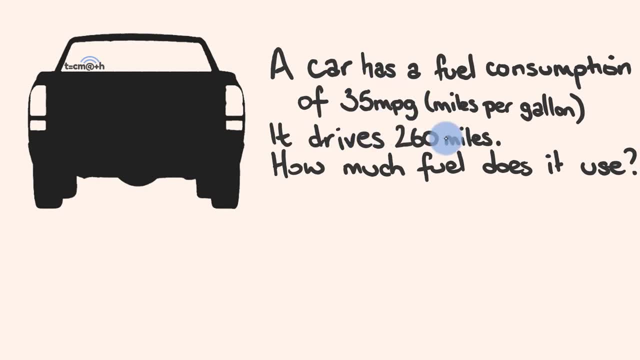 31.7 litres of petrol that we'd need. Okay, let's have a look at this involving miles. A car has a fuel consumption of 35 miles per gallon. It drives 260 miles. How much fuel does it use? So, as you can see here, we have 35 miles, and this is with one gallon. 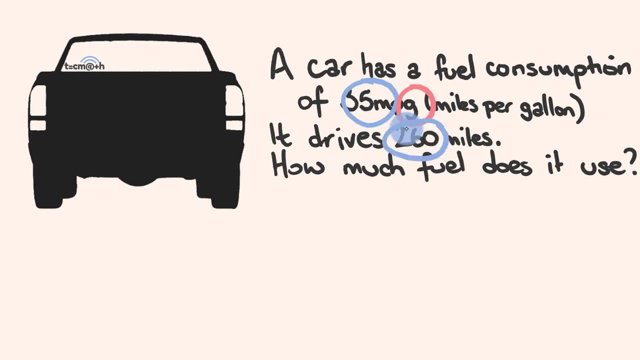 We also have a fuel consumption of 35 miles per gallon, So we're going to have a fuel consumption of 360 miles per gallon. We also know that we're traveling 260 miles, But what we really want to then find out is: how much fuel do we use? How many gallons do we need to do this? So let's write this. 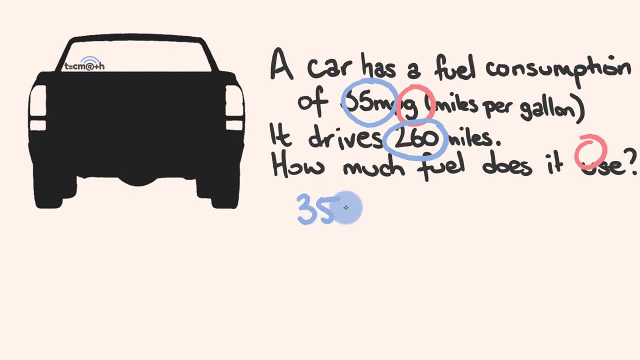 all down here. We have our fuel consumption, which is 35 miles, and that is using one gallon of fuel. We are driving 260 miles, And what we want to really find out is how much fuel we're going to be using to drive that far. So, as you can see, we're going to have a fuel consumption of 35 miles per gallon.